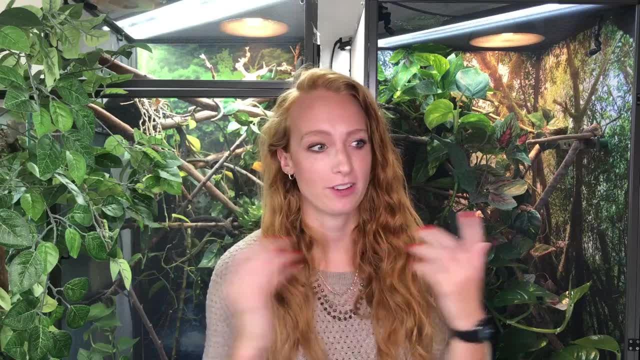 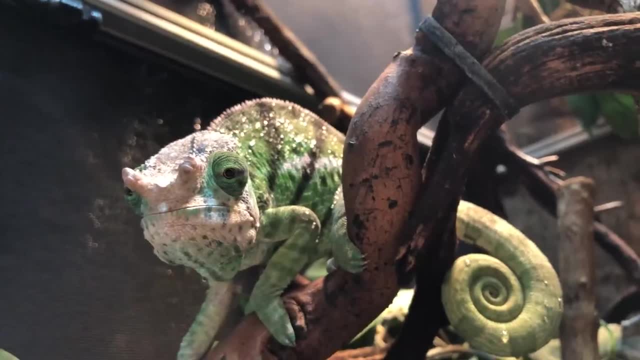 doobie roaches after I stopped offering him the super worms. But it's very easy to freak out and panic and go: oh my gosh, they're only eating super worms, so I got it. That's all the food I can offer them In the wild. the chameleon's not eating every day and 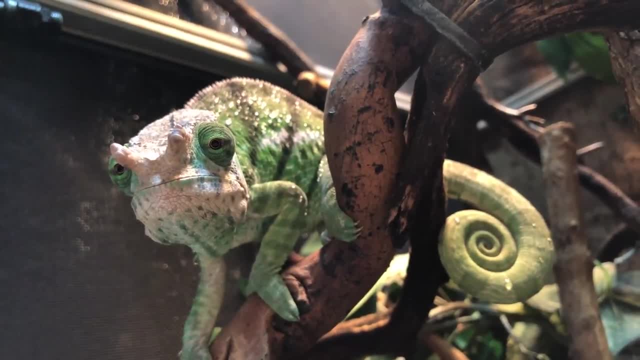 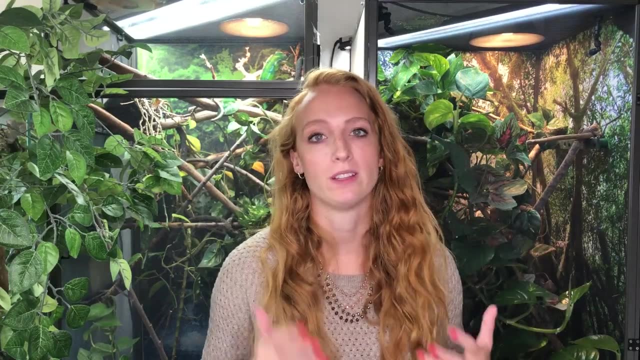 a chameleon's not going to starve themselves. So just stop offering them that and offer them the other bug. Another tip that I'll offer is to make sure that the bugs are moving. This is especially true with roaches. So say, you have an adult chameleon, and adult chameleons usually only. 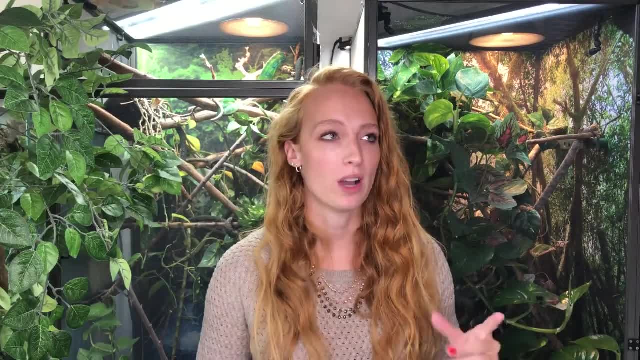 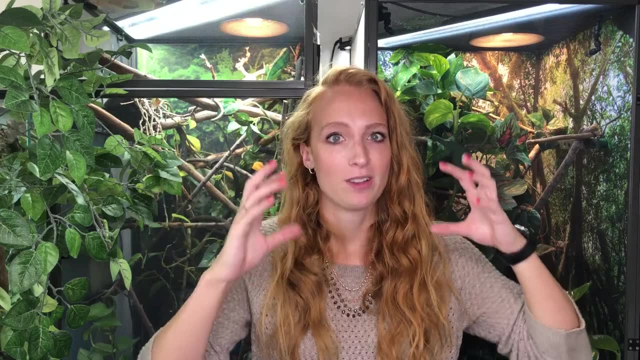 eat about three to five bugs per meal. So you're like, oh, I'm just going to put three doobie roaches in there, OK, but the three roaches are just going to run to the corners and not move. So what I'll do is I'll put significantly more roaches in there. So then, 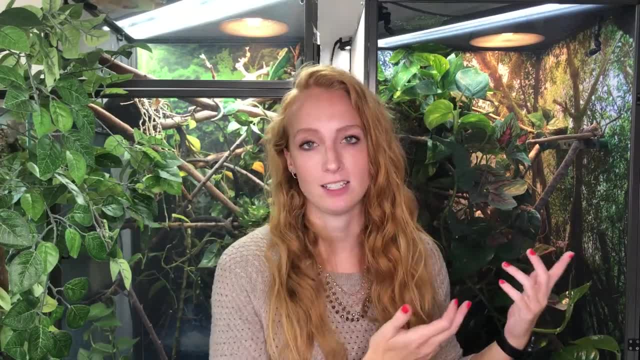 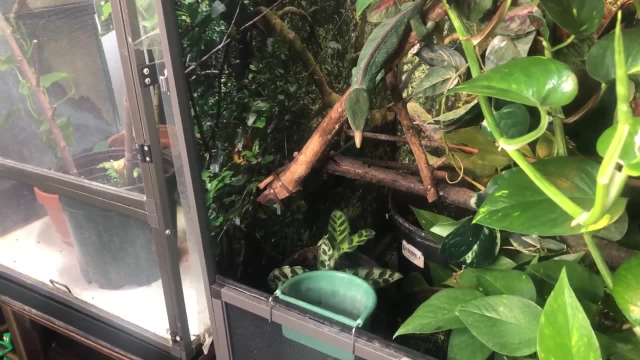 they're moving around and bumping into each other, which is going to catch the attention of the chameleon, because they're attracted. This is also the benefit of cup feeding, because then you can kind of track how much food they're eating. But that would be my advice to you. Additionally, make sure you give them privacy. 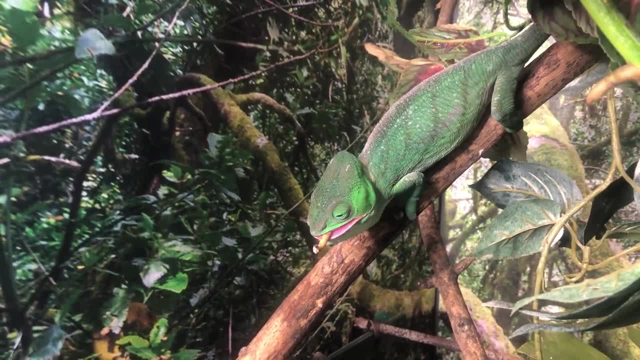 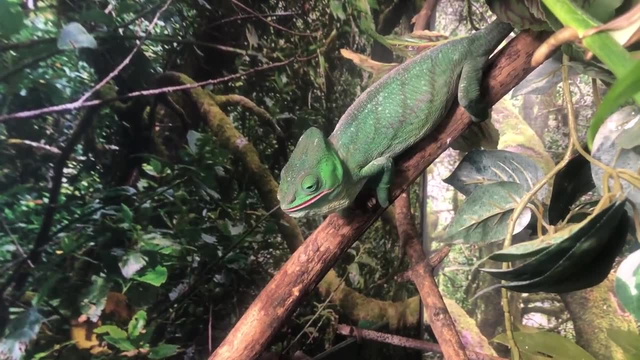 I mentioned that earlier. Chameleons are shy eaters, so make sure you're giving them space to eat their food. And sometimes chameleons are just bored of the bug and they get stubborn and they are not going to eat anything else because they turn their nose up to the crickets or the. 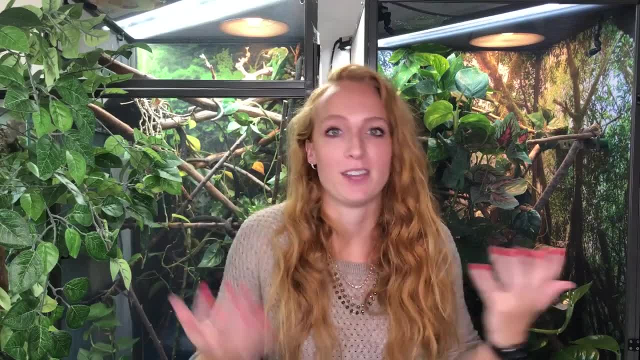 roaches or whatever it is, And you just need to offer them distance. But you also want to make sure your chameleons are not eating different types of bugs, different variety. You know humans are the same way, Don't get me wrong. 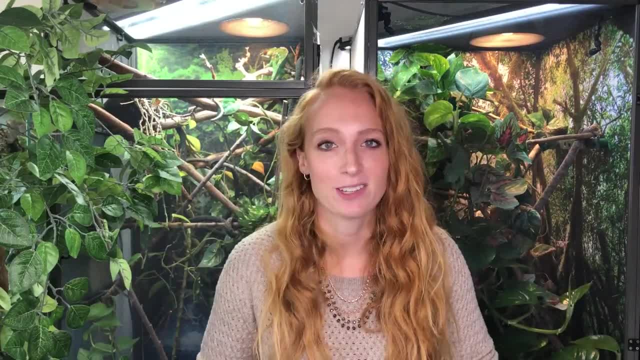 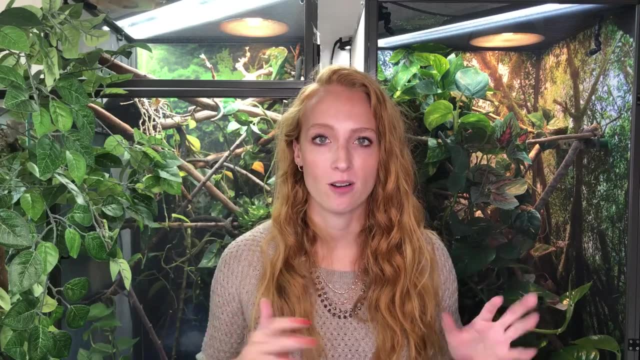 I like chicken and rice, but if I ate chicken and rice every day, I'd probably stop wanting to eat it. So make sure you're introducing variety and you're changing out your feeders and giving your chameleon different options. I have a whole video on different types of bugs that you can feed to your chameleon. 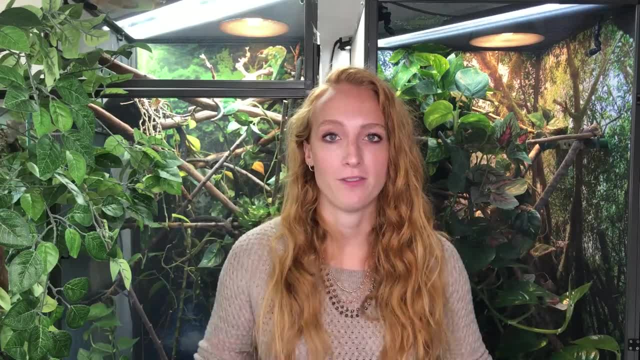 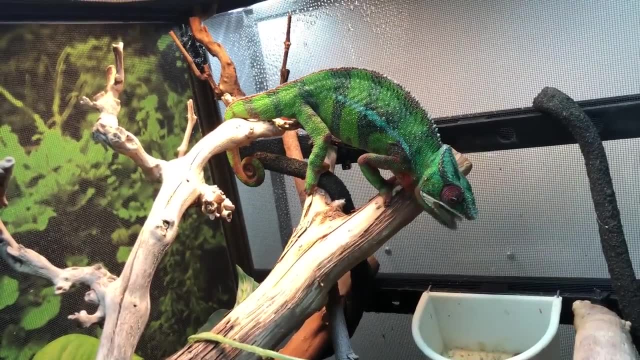 so I'll link that up above here and in the description box below And hopefully that will give you some ideas on different bugs you can try. So those are the most common reasons for a chameleon not eating. They're new, They're picky.